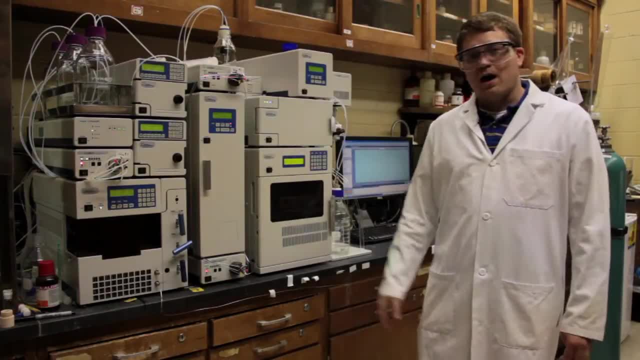 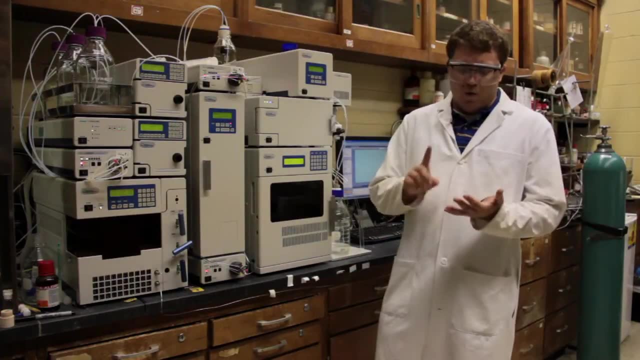 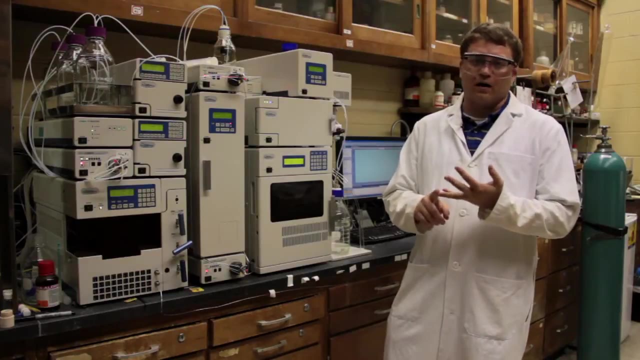 Hi, I'm Jason. I'm going to take you through an SFC. It's a supercritical fluid chromatography instrument. Here in the Smith Group we use it for three different things: One for normal chiral analysis, Two for chiral separations of medicinal chemistry targets And three for separating compounds for diversity-oriented libraries. 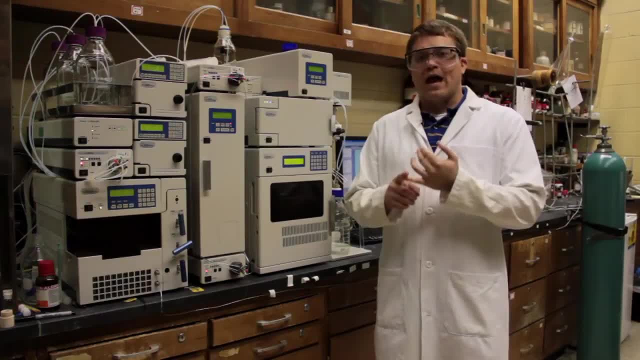 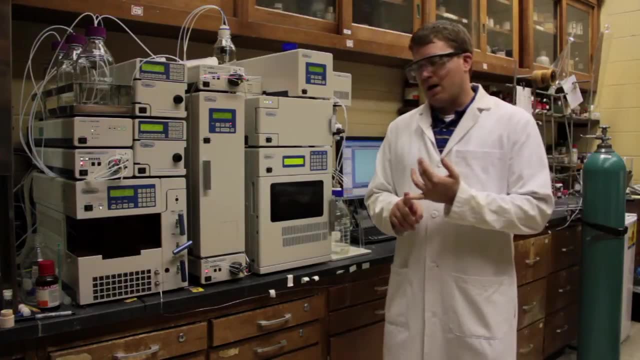 Number one. when we run reactions here in the group, this is a very fast tool for figuring out whether or not we got the EEs that we'd hoped to. The run times on a supercritical fluid chromatography instrument are significantly shorter than a normal HPLC. 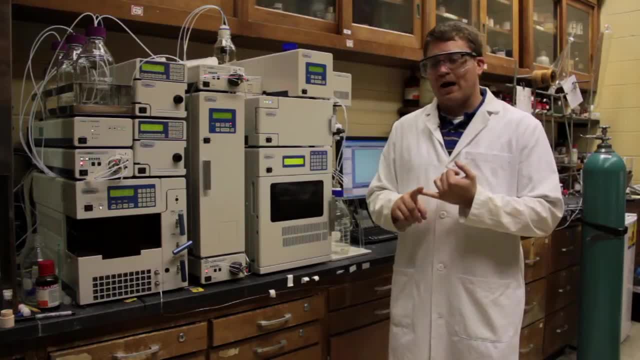 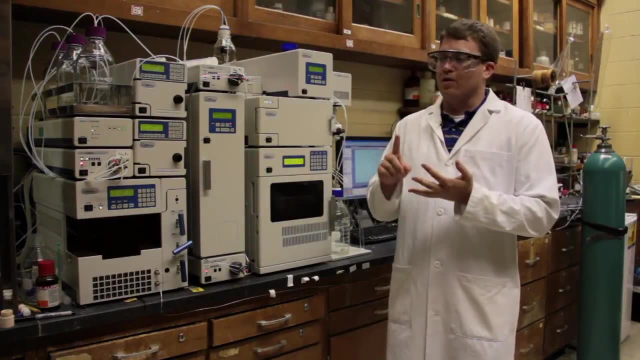 A normal HPLC's runs would be somewhere in the range of about an hour. These runs are about 10 minutes, So in the time to screen columns even for this it would take overnight probably. on a normal HPLC We can do it in about an hour, So that's really really sped up our analysis time when it comes to running chiral reactions. 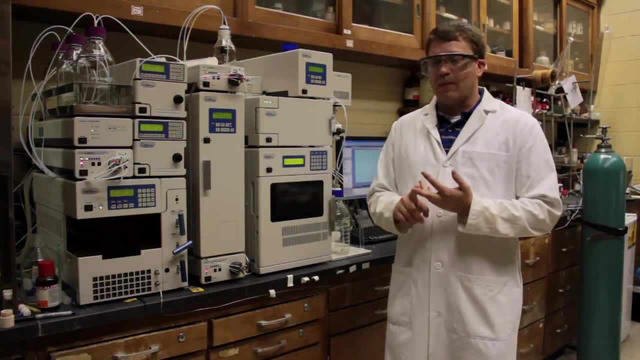 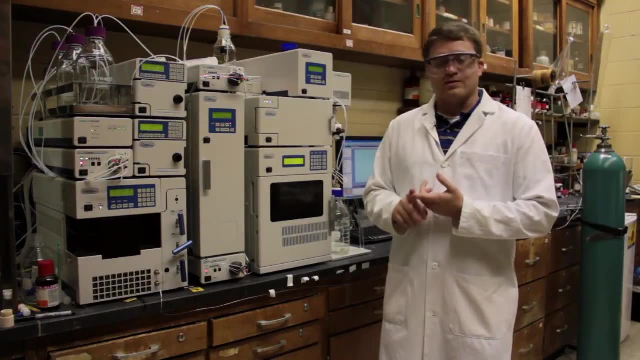 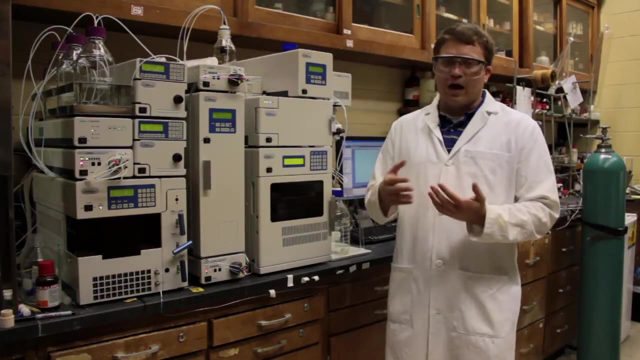 Secondly, we have quite a few collaborations here in the Smith Group with biological groups to work on medicinal chemistry projects, Because the targets we're working on are chiral. often times we need to figure out whether or not which of the enantiomers of the chiral reactions we're going to be working on. So we're going to have to figure out which of the enantiomers of the chiral reactions we're going to be working on. So we're going to have to figure out whether or not which of the enantiomers of the chiral reactions we're going to be working on. 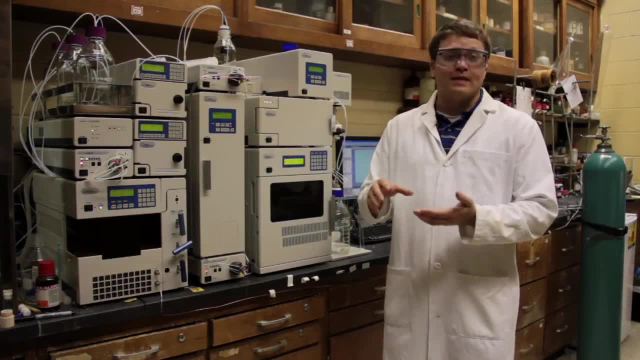 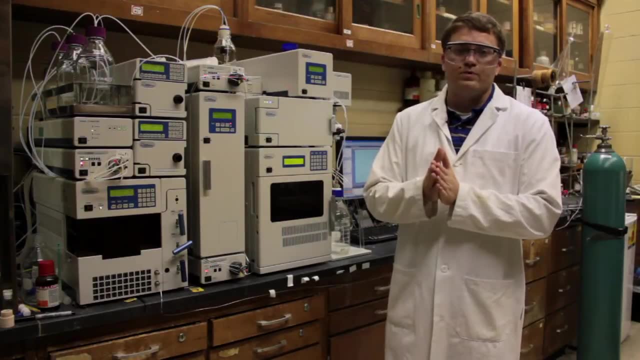 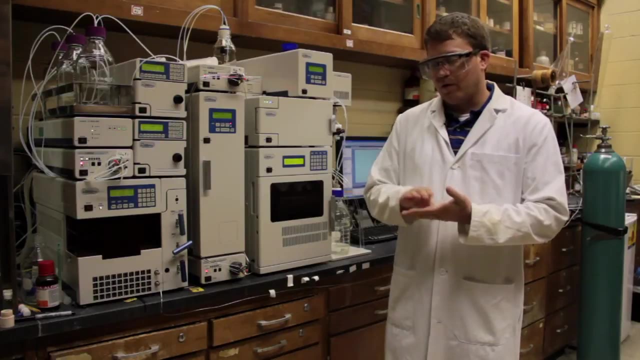 So in the area of the compounds that are actually inhibiting, the target is the active one. So we have used this- because we have a semi-prep mode on this- to actually separate upwards to 2 to 3 milligrams of each enantiomer for testing. 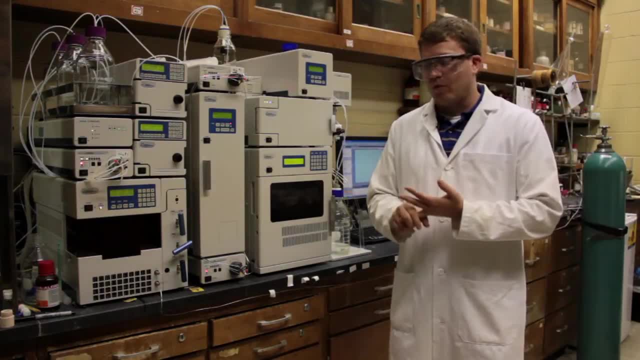 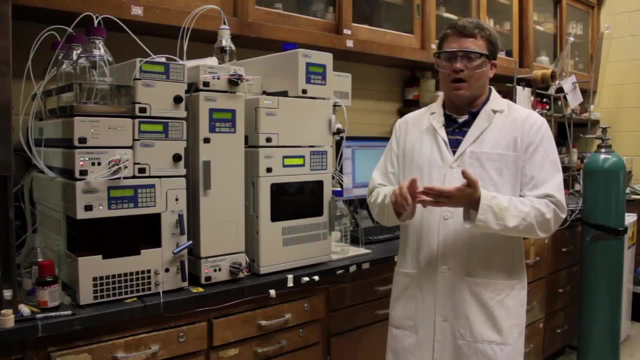 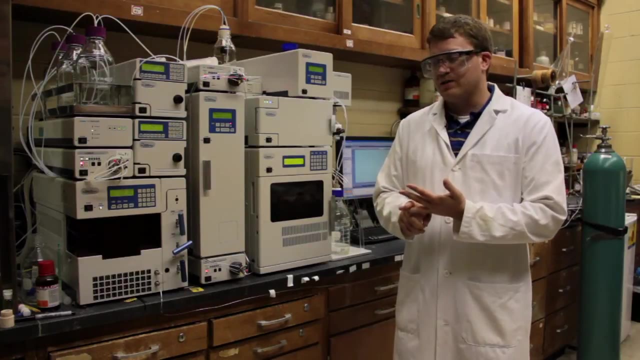 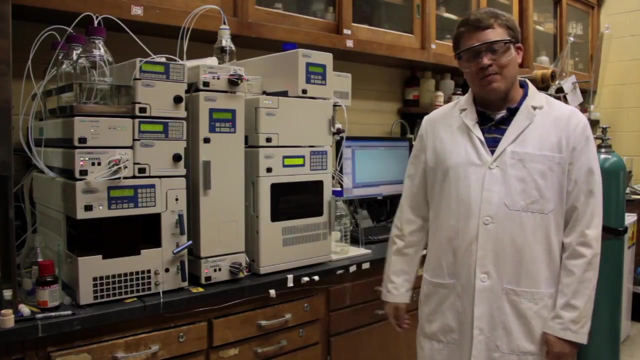 The other thing we use this for is for utilizing one of the methods we developed in the group, our chemistry, And this has been instrumental in separating many of the diastereomers in that project. My name is Jason Melvin. I'm a fourth year graduate student here at the University of Pennsylvania in Amos Smith's lab.